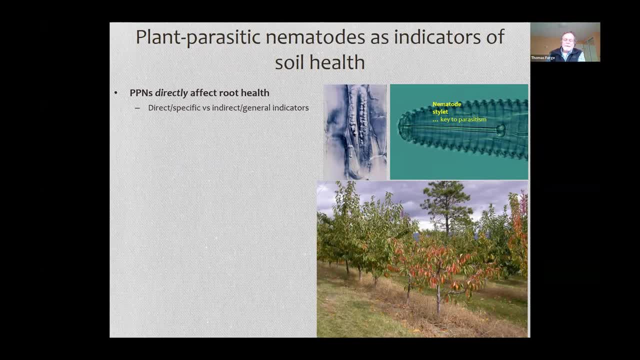 on root health, And so for this reason they're good indicators And we also know that they're widespread, And so for something to be useful as an indicator it needs to be fairly widespread and present, you know, in most places. But they vary at, but they exist at variable population. 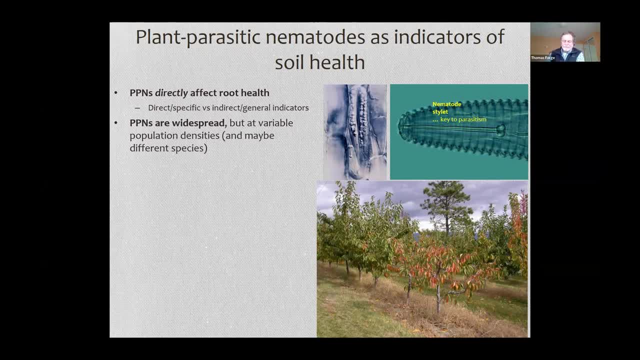 densities depending on where you are, And so that also kind of adds to their value. you know if that variation in population densities is related to the broader question of soil health? And so even though they do directly affect root health at the scale of orchards and variation, 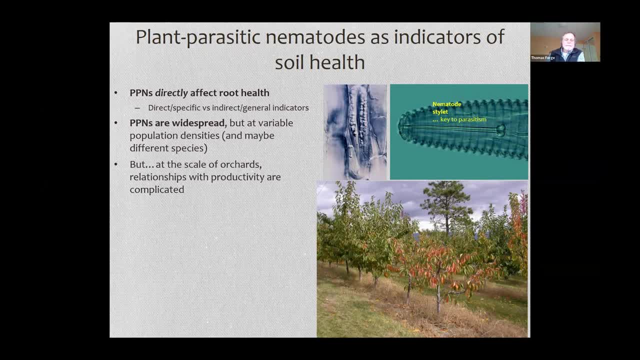 among orchards out on the landscape. those relationships with productivity are complicated And we'll dive in a little bit more detail about this later on. But just you know, to very quickly go over it with nematodes there are no obvious signs or symptoms such as certain other types of. 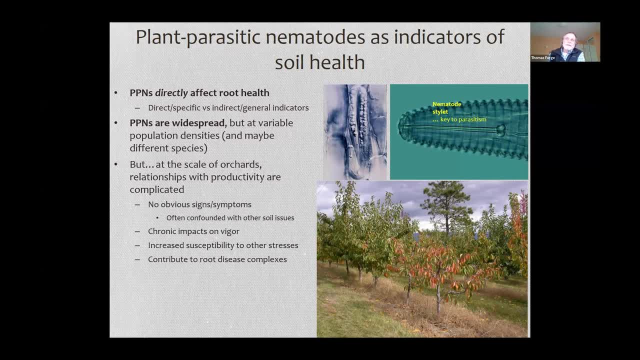 diseases And they, the populations, often get confounded with other soil stresses, which is part of the reason we look at them as a problem And so you know we have to be very careful about as part of the broader question of soil health. But it also adds to the difficulty in relating 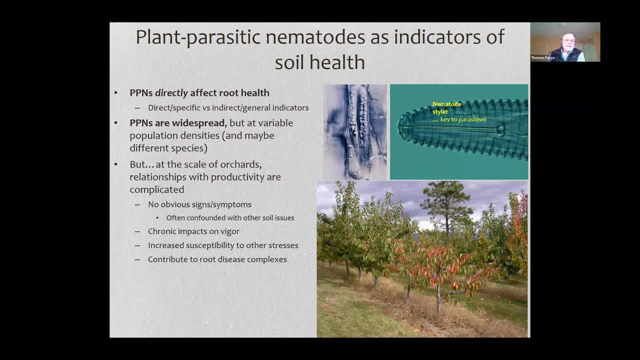 their populations to overall productivity and yields and packouts and what have you? And? but nematodes do have long-term sort of chronic stresses on vigor. even though they don't really take trees down on their own, They increase susceptibility to other stresses And they also 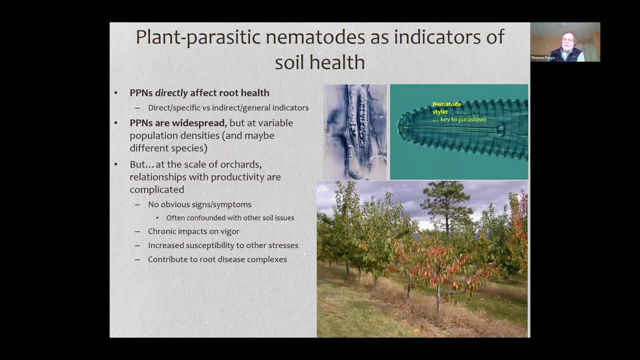 contribute to root disease complexes. So there are, as everybody knows, there are other fungal pathogens out there And in the process. there are other fungal pathogens out there And in the presence of nematodes, these things kind of come together in a little bit more extreme fashion. 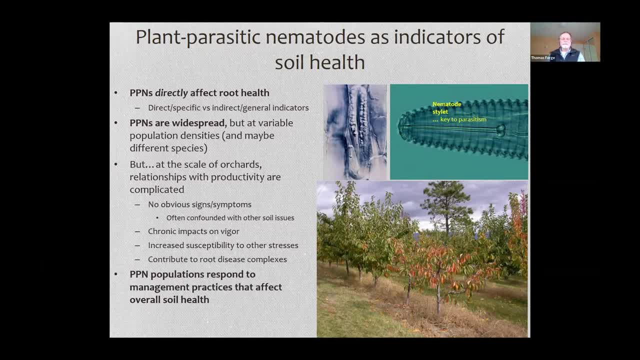 And but also plant parasitic nematode populations themselves respond to the management practices that affect overall soil health, And so in this way they're also indicative of broader changes in the soil. So we'll dive into this in a little bit more detail. 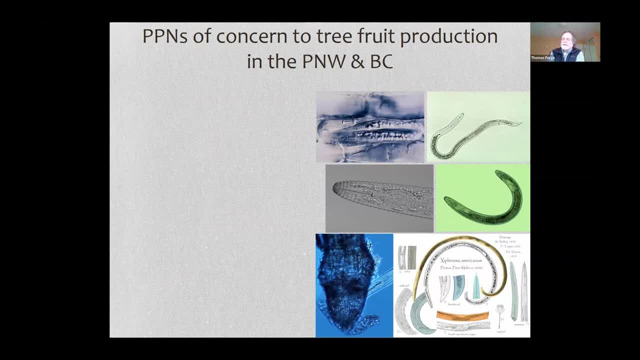 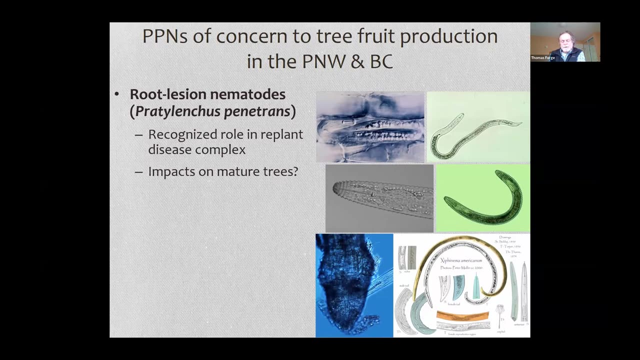 So the plant parasitic nematodes of concern to tree fruit production in Pacific Northwest and British Columbia. foremost is the root lesion nematode, Pratylencus penetrans, And you've heard all about this nematode, I'm sure many times before, And we'll spend most of the rest of this presentation. 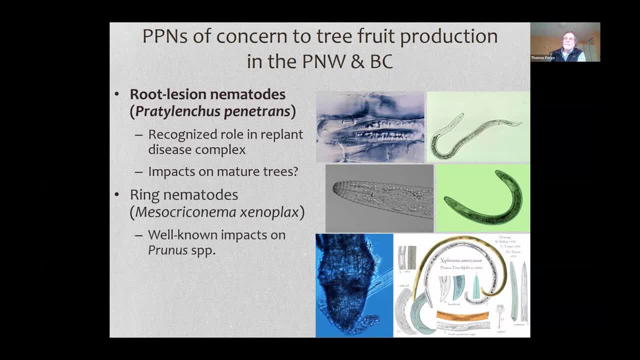 talking about that nematode, But I do want to point out that there are nematodes of interest to tree fruit production in the Pacific Northwest and in Canada, in British Columbia, And one that has really kind of come up more and more on our radar is the ring nematode or mesocrichinemma. 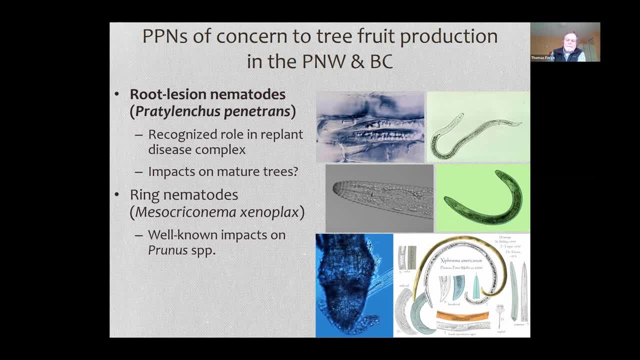 xenoplax. This nematode is not an issue on apple, but it potentially is an issue on cherry, And we're trying to work this out. It's well known to be an issue on peach and plum in places like California and the southeastern United States, And I'll talk a little bit more about this. 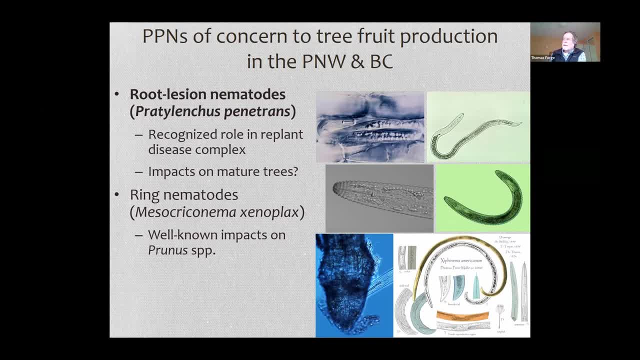 And we're just starting to learn. we're starting to find it more and more in cherry trees And we're starting a little bit more about it. Dagger nematodes are not directly important in that, you know, in most cases their population densities in our region are not high enough to 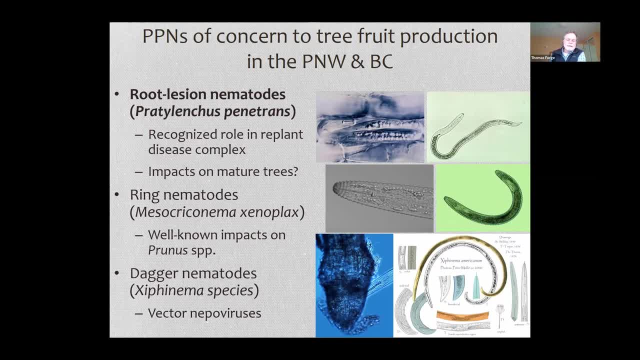 directly cause damage, But they are really important to keep in mind and to be aware of because they vector Nipah viruses, a particular class of viruses. Tomato ring spot virus is one. tobacco ring spot virus is another. cherry rasp leaf virus is another. 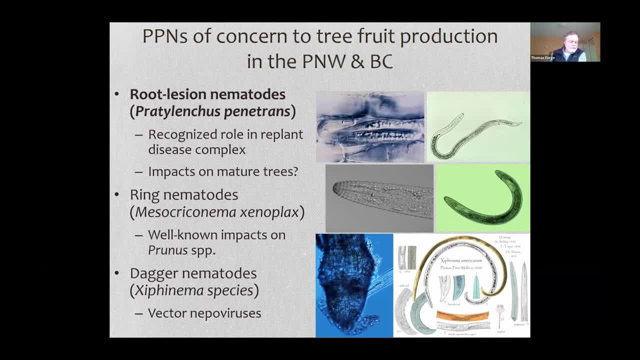 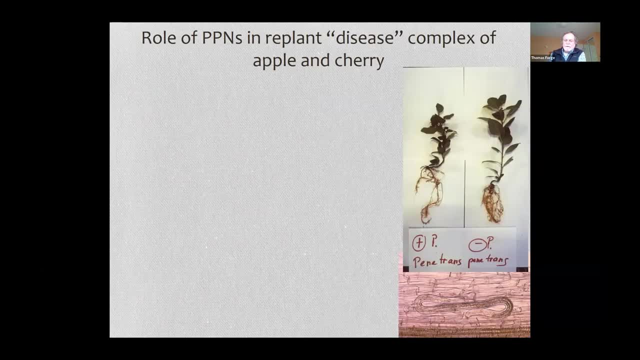 yeah, I'll go into these a little bit more, But you're not quite sure that- and so if these viruses get into your orchards, it's very important to know whether you have these nematodes and what population densities. So most of what we know about the impacts of plant parasitic nematodes on fruit trees is limited to. 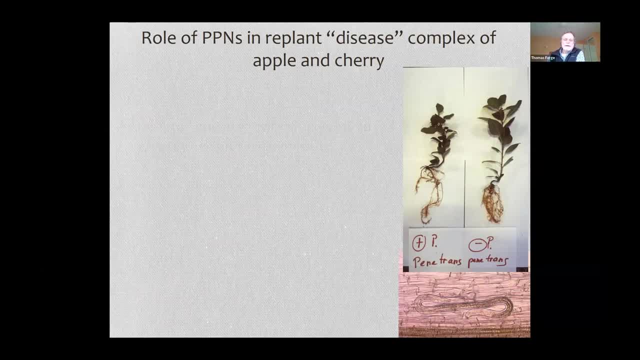 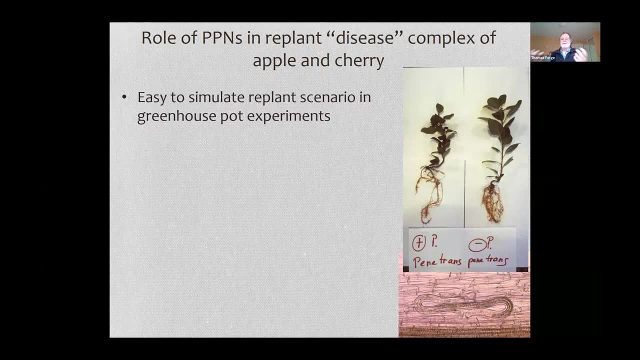 the role in replant issues, And there's a very good reason for this. It's very easy to simulate the replant scenario in greenhouse pot experiments, in which you can have an apple seedling and you can grow it in the presence of nematodes right next to one growing in the- without nematodes in the. 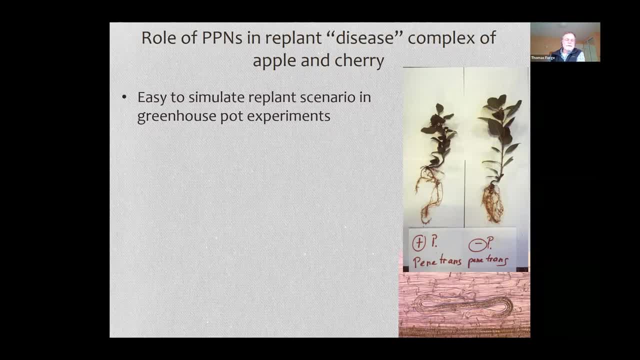 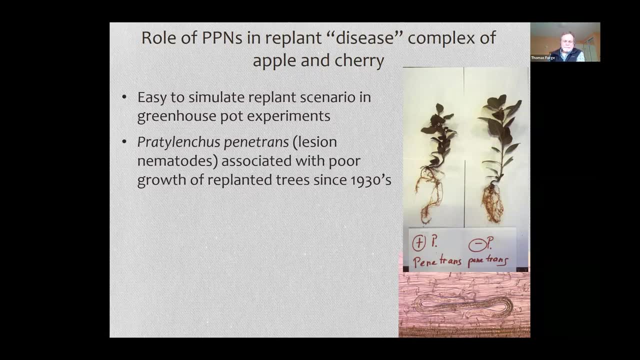 nematodes and then compare the growth of those seedlings. So it's very easy to demonstrate the influence of nematodes, essentially their pathogenicity, And in this context the root lesion nematode has been associated with poor replant growth of apple trees since at least the 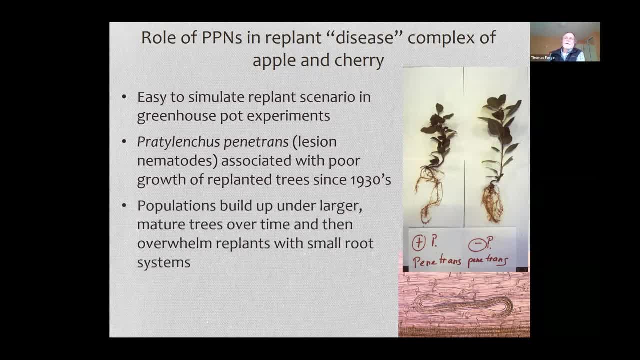 1930s. I think is the earliest report I've ever seen. After World War II, of course, with the advent of widespread fumigation and availability of fumigants, we became a lot more aware of the role of these nematodes in replant issues, And what happens is in longer established orchards. 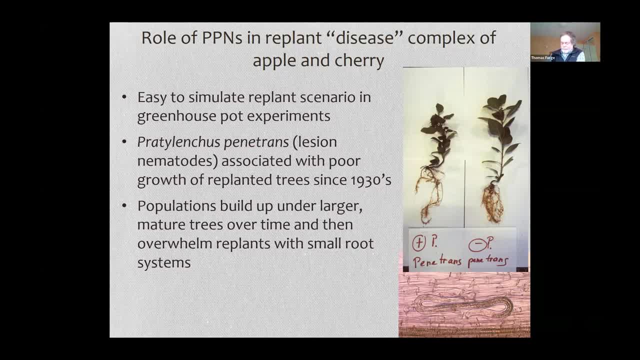 large trees, large root systems. these populations build up through time And then when you go to replant with these little seedlings, small trees, with small, limited root systems, there are just too many nematodes and they overwhelm the root systems. And the other point I want to make: 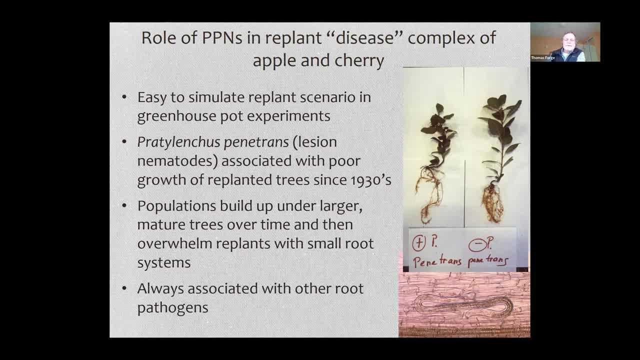 very clearly is that in replant scenarios, these root lesion nematodes are always associated with other root pathogens: Rhizoctonia species, Fusarium species, Pythiums, Ancylindrocarpin or Ilionectria species. 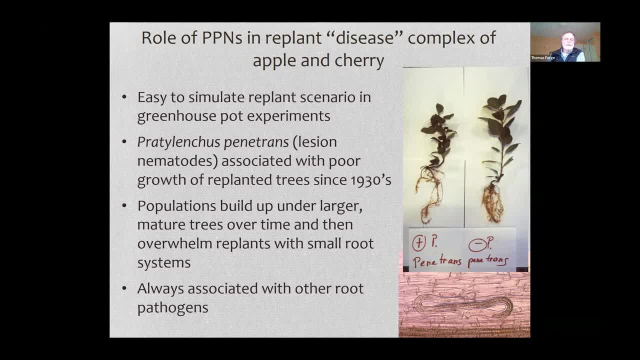 And so it's important to be aware of that- that nematodes aren't the only pathogen in the soil, but they play a particularly important role because they themselves, as they burrow into roots, enhance susceptibility of roots to some of these other pathogens. 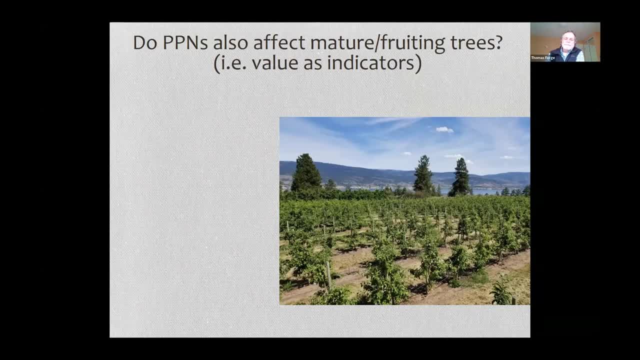 So one of the interesting questions from a soil health perspective is: do plant parasitic nematodes also affect? you know, have direct effects on mature or fruiting trees. And the reason I bring this up even as a question is because sometimes, when we were so focused on the replant scenario, 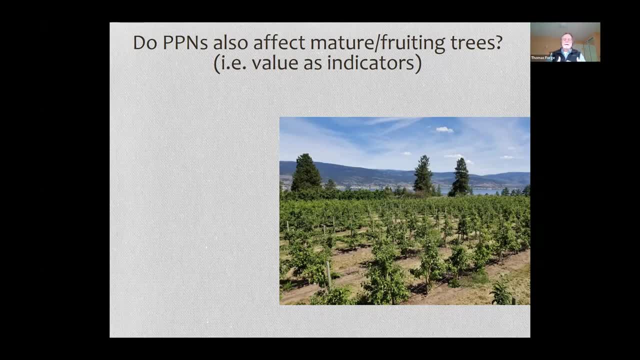 and we talk, and we get focused on it and we talk about, you know, doing management practices to minimize, such as fumigation or what have you, to minimize population densities at the time of planting. And if we can just protect those nematodes, we can do that, And so I think it's. 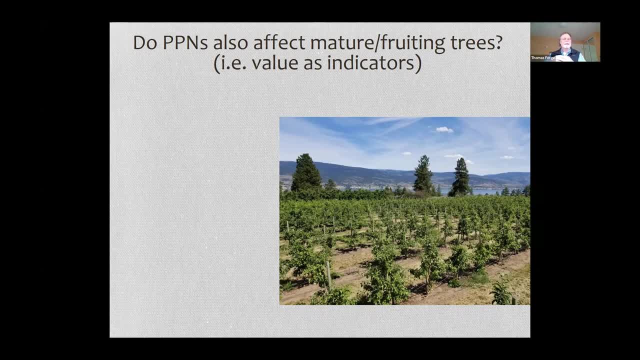 very important to be aware of that. I think if we can just protect those nematodes, we can do that. And then we often kind of wipe our- you know, brush our hands and think: well, you know that once a tree is established they can probably withstand nematode populations, And this is kind. 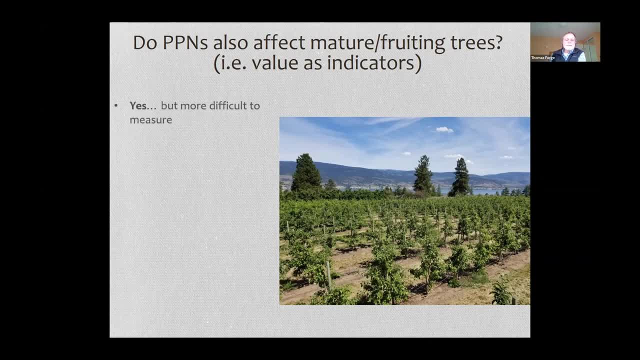 of a. it's almost a conventional wisdom that's been put out there, But in fact, I mean, these are parasites. they are still building up in their populations on established trees And so, yeah, I think we can say yes, they are affecting mature fruiting trees. 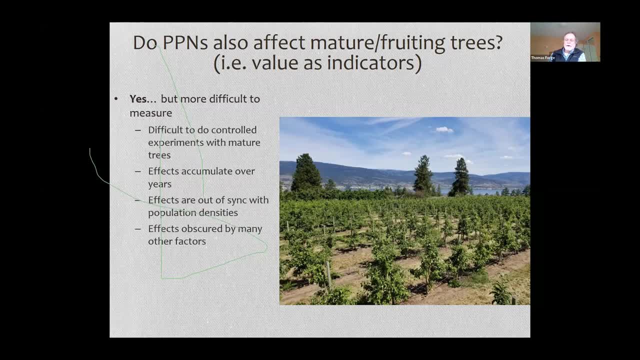 But it's very difficult to measure, which is why we do not have a lot of strong information on it. As kind of similar to what I was indicating before, it's difficult to do controlled experiments with mature trees compared to, say, greenhouse pots. 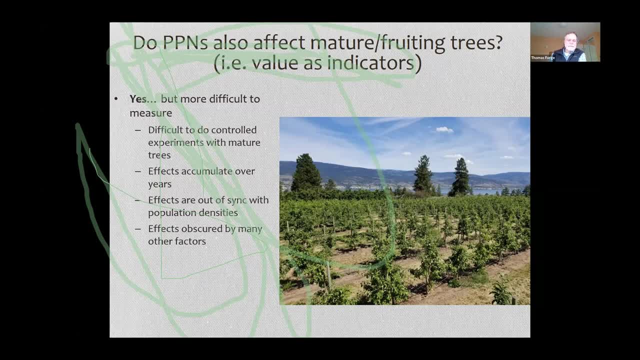 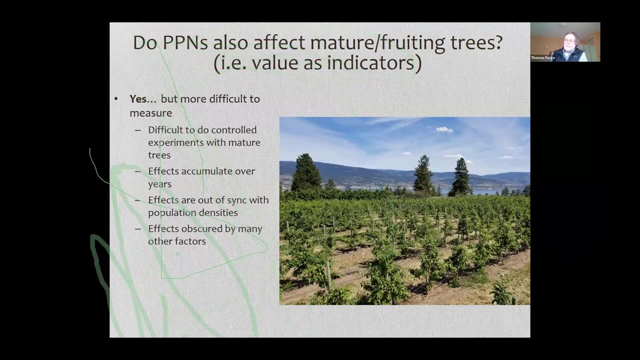 Effects accumulate over time on a long-lived perennial crop. So feeding in this year and nematode feeding in the next year will impact growth and productivity five years down the road And similarly the effects. because they accumulate like this, they're out of sync, often with population densities. 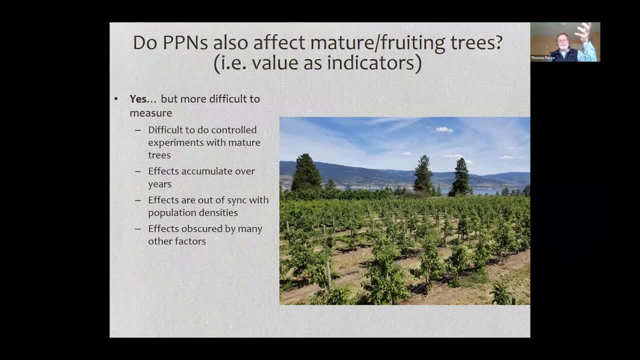 So if you're measuring population densities now but the tree, the status of the tree, is reflecting population densities that were three years ago or two years ago, then very often you don't get a. you know it's difficult to get a good quantitative relationship between population densities and the way the tree is performing. 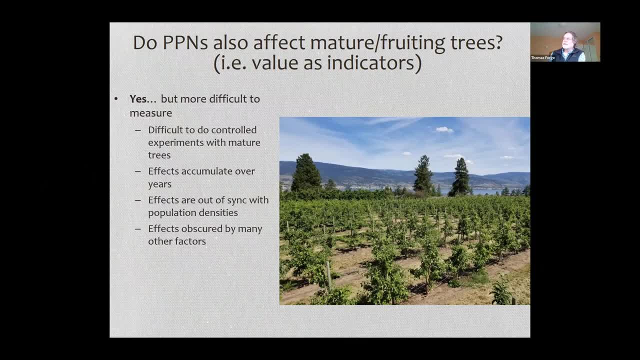 And, of course, being out in the field and in relation to other pathogens and things like that. as I mentioned, in general the effects can be obscured by many other factors that are also affecting the trees, But nonetheless there have been a few studies that have successfully correlated or related in some way, sometimes a very complex statistical models. 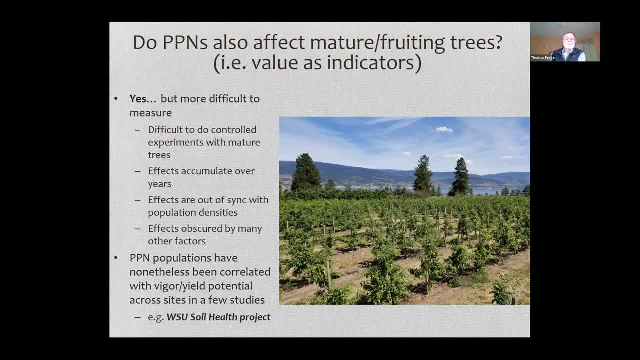 but they ultimately correlate the vigor or yield potential across sites with population densities of root lesion nematodes And so, like, this project that Tiana has been working on and was just describing is one example of this, And so this is kind of underscores the value of this kind of work, this soil health work. 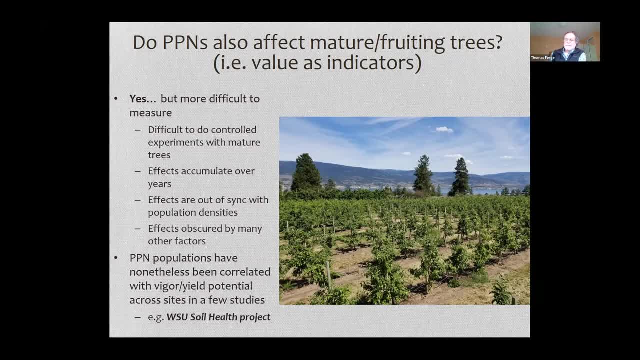 also leads fundamentally to a better understanding of the relationship between nematodes and productivity out on the landscape. And before I leave this topic of the mature fruiting trees, I'm just going to throw out a food for thought. I've always been curious about the role of nematodes in these high density planting systems. 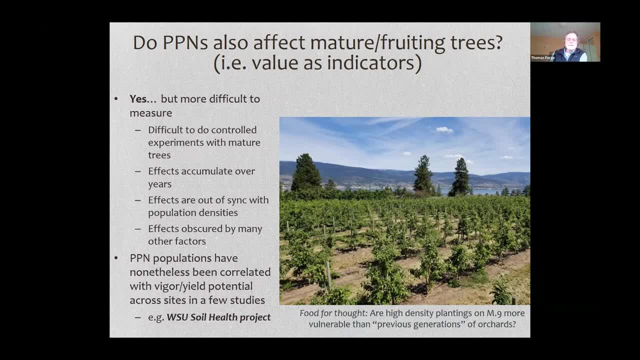 vis a vis the good old days, so to speak, where we had large trees with very robust root systems, and I can't help but wonder if these systems are more vulnerable than the previous generation of orchards. and it's difficult to do that kind. 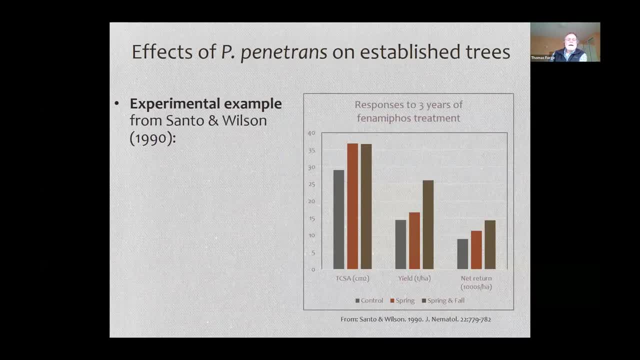 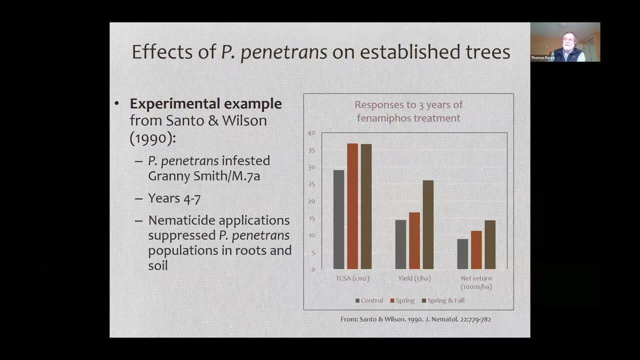 of experiment, because the whole system has shifted through time. So I'm going to provide one of the few experimental examples of the impact of nematodes on established trees that I know of or that I've been able to find, and this is Jerry Santo down in Prosser, way back in the mid-1980s. 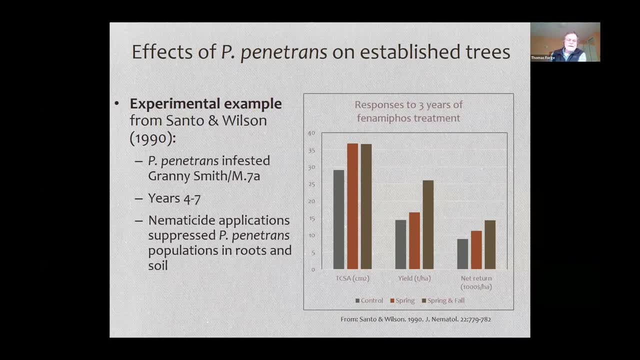 He did this work and it was a site that had p-penetrans and the site was Granny Smith on M7 and in years four through seven of this planting- so not super mature trees but at least you know- established and fruiting- Jerry went in and applied a nematicide that we no longer have available. It's 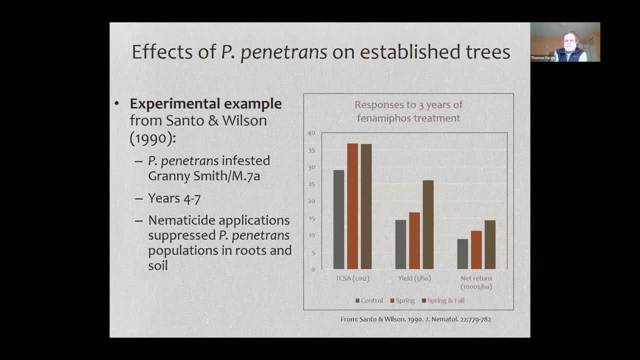 called Phenamifos or Nemacure. It was a very effective nematicide and it's fairly specific and he applied it and succeeded. He successfully suppressed the nematode populations and, I should point out, he did a spring application as well as a spring and fall split application, which is why there 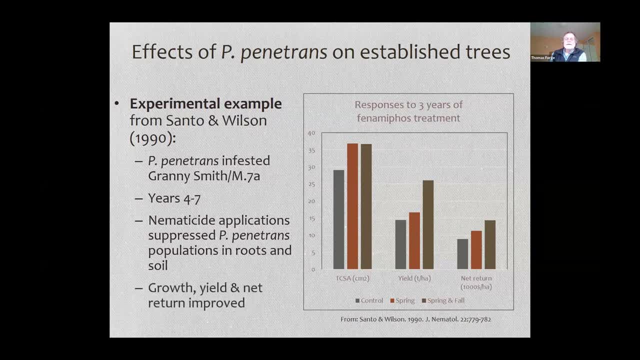 are three different bars on that graph- but basically, and so he was able to suppress the nematode populations and in response, he got improved growth yield and net return productivity. and so this is, you know, one of the few examples from a field experiment in which nematode populations were manipulated and there was a corresponding improvement. 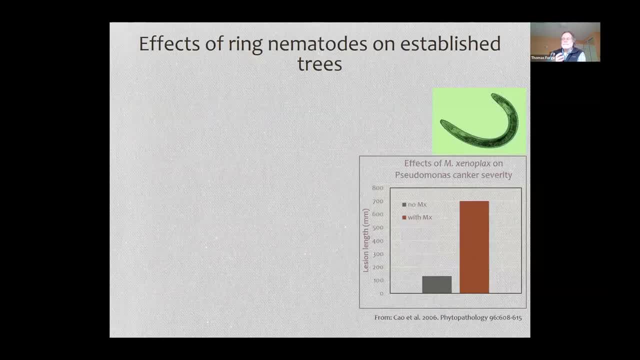 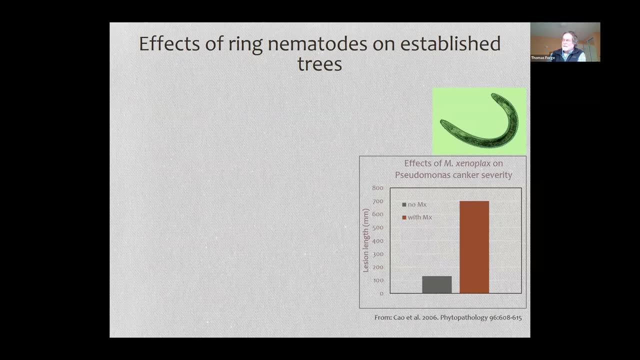 in growth of the trees- Not that I'm saying that we should go back to using Nemacure or anything like that, but it also illustrates how sometimes these chemicals can be good experimental tools to help us understand something. Another example of the impacts of nematodes on established trees: 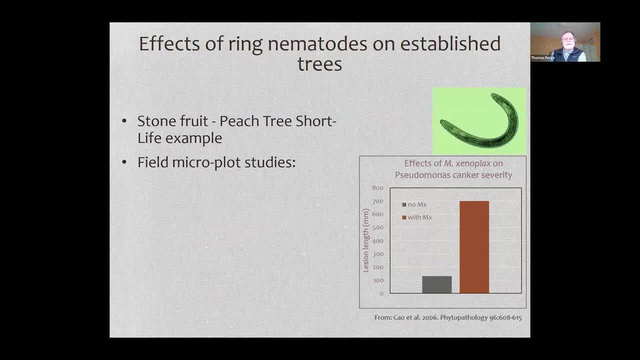 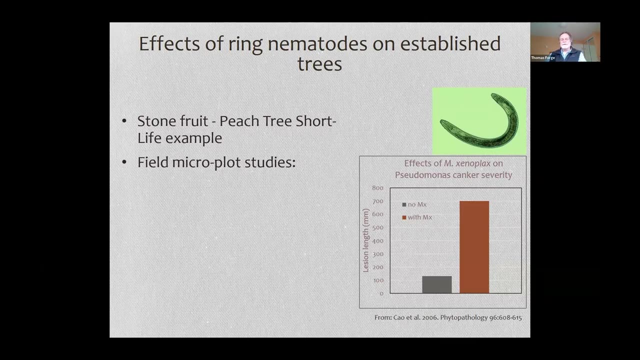 comes from the stone fruit ring nematode situation. There's a disease complex called peach tree short life, and these nematodes play a very important role in it. A lot of work has been done using an approach we call microplots, where there are large chambers out in the field. 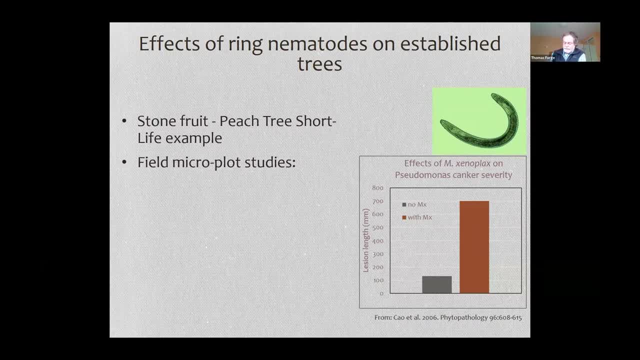 where the soil is fumigated and then re-inoculated with the nematode, so you can control whether the nematodes are there, just like a greenhouse experiment, but it's just much bigger and more complex because it's out in the field. 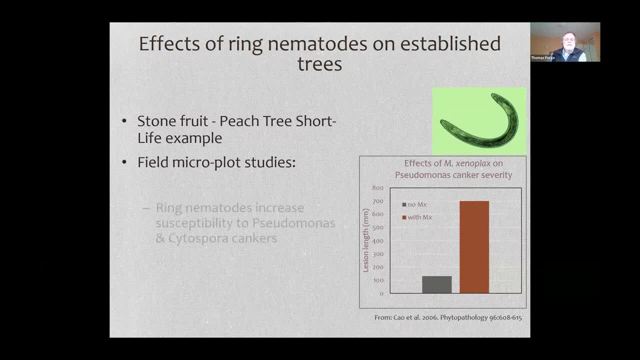 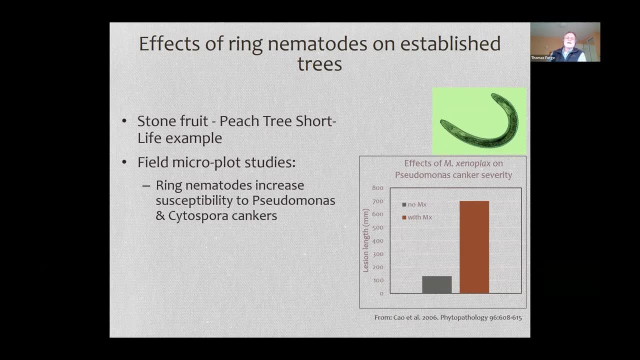 And grow the trees up to a decent size, and so what a number of researchers have found is that the presence of these nematodes increases susceptibility of the trees to Pseudomonas and Cytospora cankers, and the graph shown down here is a graph of the size of the lesions. 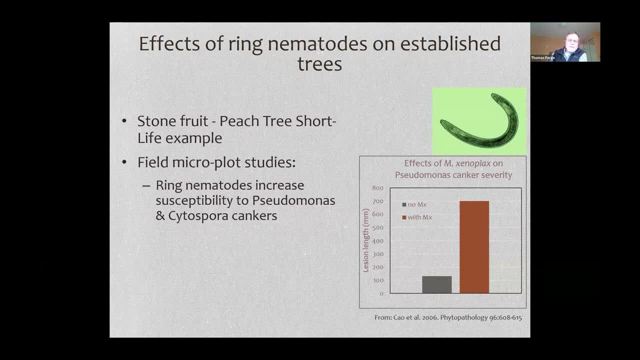 for trees that are growing in microplots, with or without these ring nematodes, and so you can see that, in the presence of the ring nematodes, the lesions caused by a re-inoculation with Pseudomonas are much larger, and so this is a really interesting example of 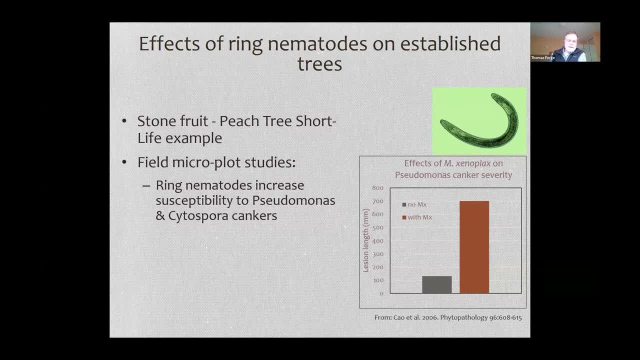 how it's kind, of these indirect effects, if you will, of the impacts of nematodes on production. Now, this is just an example. I throw this out there. No similar work has. well, first of all, ring nematode doesn't go to apple, but even in the context of other nematodes such as Pradalinkas, 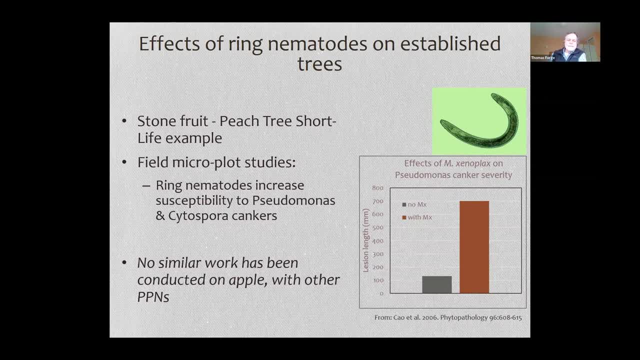 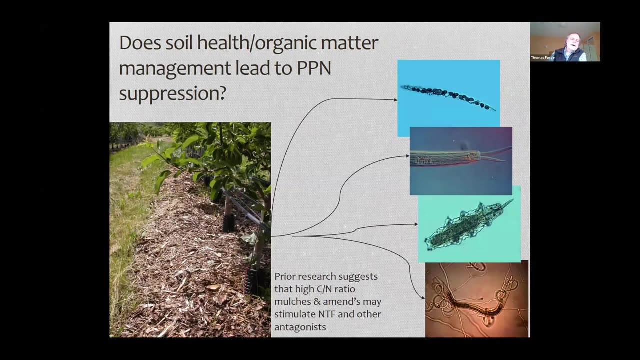 this type of experiment has not been done, and I think is something that would be useful to do in the future to help us understand these more new, nuanced influences of nematodes on trees. So now I'm going to shift in kind of the second half of what we're talking about, which is, how do management practices? 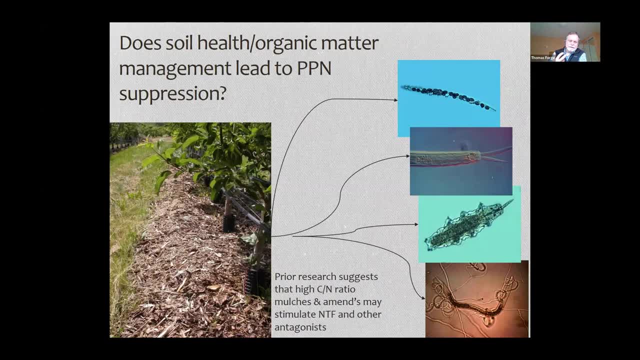 that are intended to improve soil health and intended to increase organic matter inputs and improve soil health. how might they lead to plant parasitic nematode suppression or regulation of their populations? And the basis for this, why we even look at it- is because, and just so that you're aware, there are a number of types of natural enemies of nematodes. 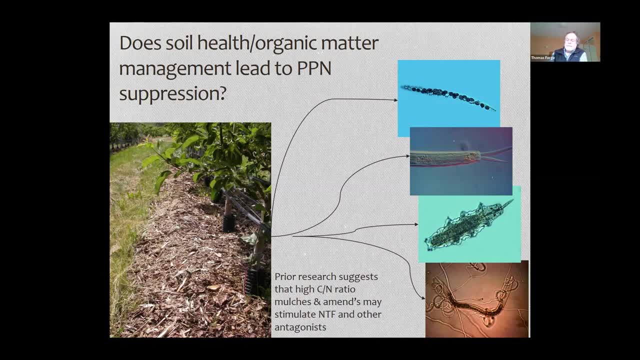 that exist in the soil. Naturally, there are nematode trapping fungi, fungi in the soil that literally create these little adhesive knobs or loops that nematodes get caught up in, And that's what that picture on the lower right is. There are other microinvertebrates, such as tardigrades. 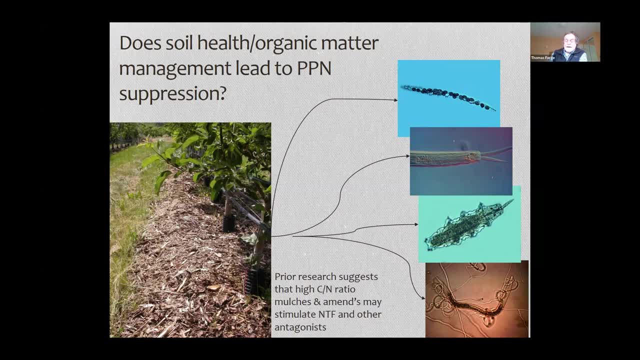 this little bear looking creature there that's actually related to a nematode that eat other nematodes. There are predaceous nematodes, as Tiana mentioned before, And so the third one up there is a predaceous nematode. 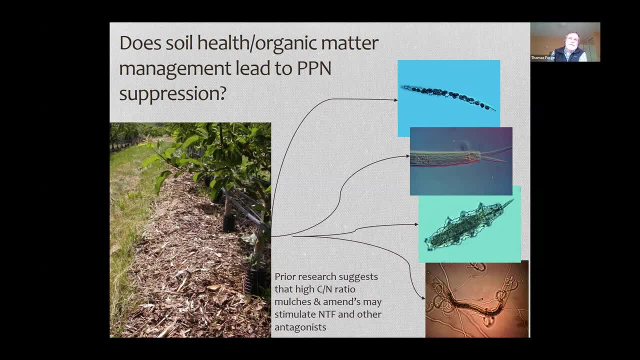 The predaceous nematode eating another nematode, And there are fungi that actually colonize, that are endoparasites of nematodes. So these are just examples of the multitude of natural enemies, And there are mites and microarthropods as well. 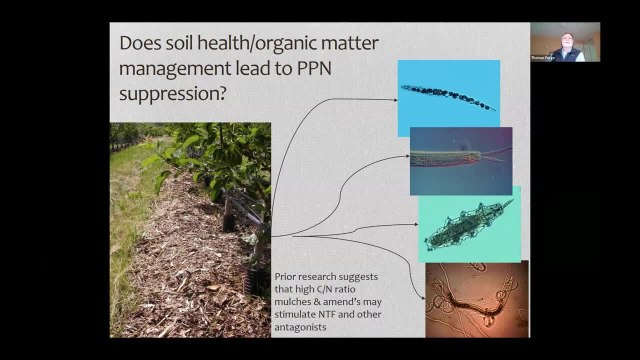 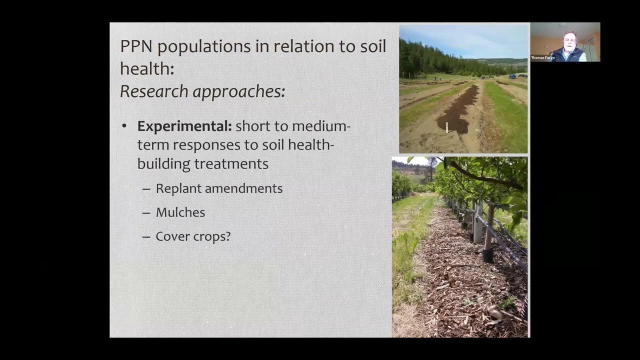 So the multitude of natural enemies, And the basic underlying idea is increasing soil organic matter inputs. in different ways, Do you stimulate growth of some of these natural enemies in such a way that it has a regulatory effect on the nematode populations? And so we've been working on this for a long period of time, a lot of nematologists globally. 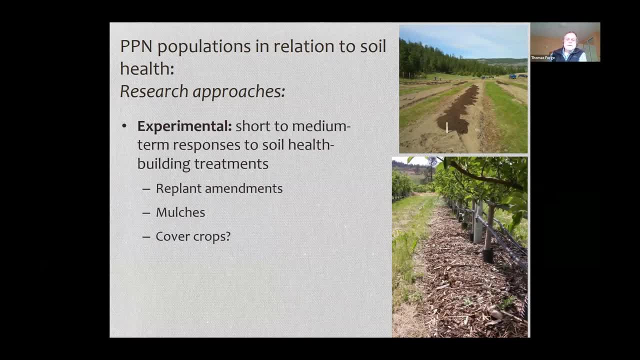 There are experimental approaches in which we set out experiments such as David described earlier- mulches, organic amendments etc. And then we monitor or measure changes in lesion nematode populations and corresponding changes in populations of these natural enemies to see if there's a connection there. 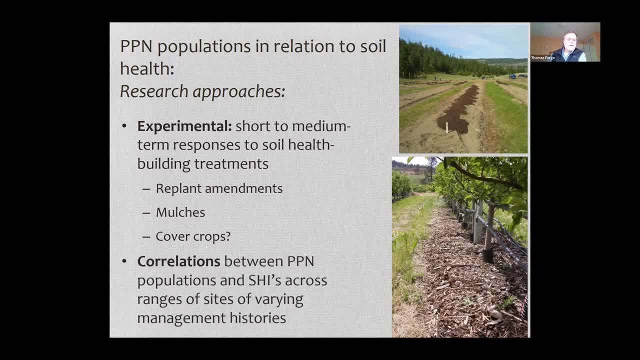 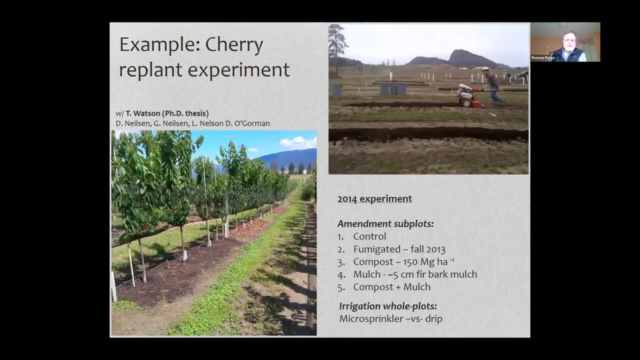 But then also, similar to the soil health, we can look at correlations between plant parasitic nematode populations and soil health indicators, or perhaps populations of the beneficial organisms across a range of sites of varying management. So I'm going to kind of give you some examples using different approaches. 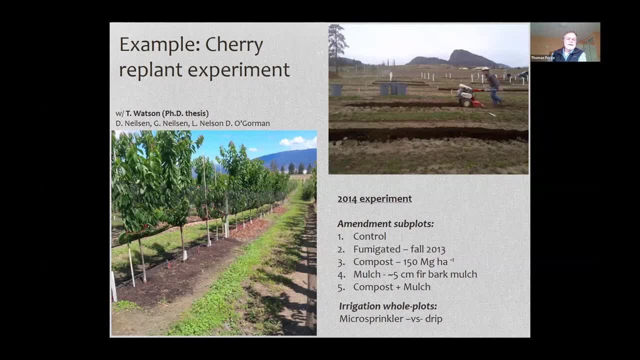 to appeal for the degree of nematode suppression that we can relate to organic matter management. The first example comes from an experiment we did up in BC. It started a number of years ago. In 2014,, we went into an old apple orchard and tilled up just the rows. 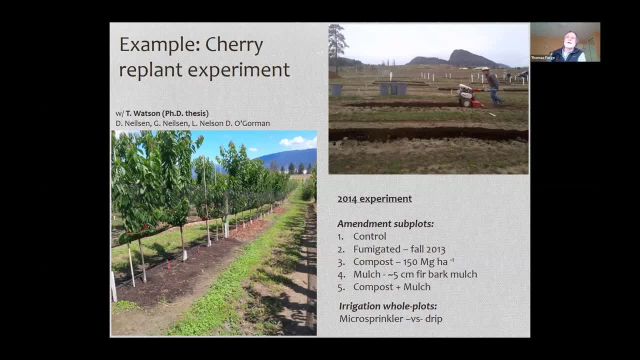 and went right back into the rows of the old apple orchard. So it's kind of a worst-case scenario from a replant perspective. But we split those rows up into five different plots. We had a control where we didn't do anything. 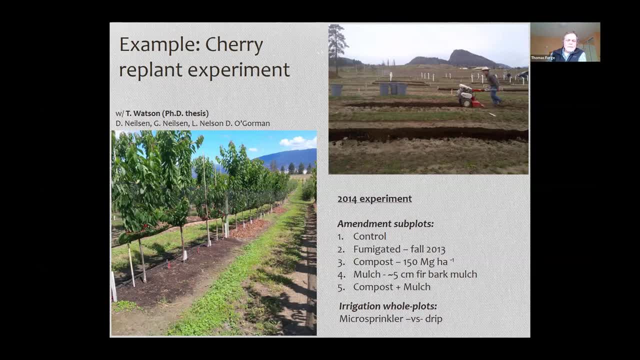 Fumigated was sort of our positive control. One set of plots: we incorporated compost at 50 dry tons per hectare. Another one: we put on a thick bark mulch right after planting, And then of course we had a combined treatment as well. 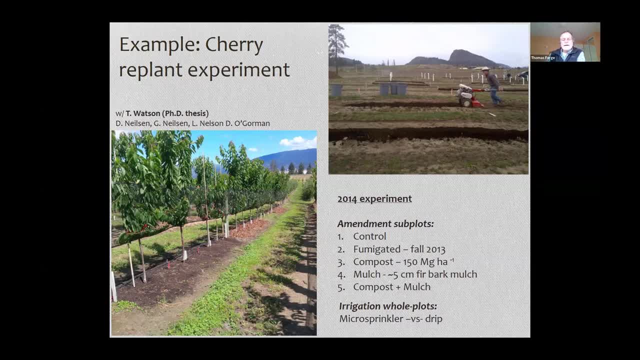 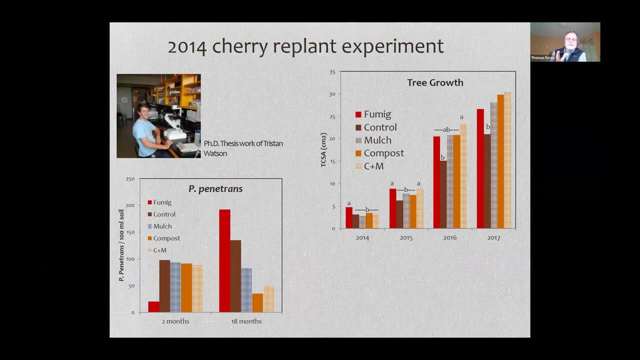 And we had multiple rows, some of which were microsprinkly irrigated and some of which were drip irrigated, which I won't get into that aspect of it, But just to quickly give you an example, just from a nematode management perspective. 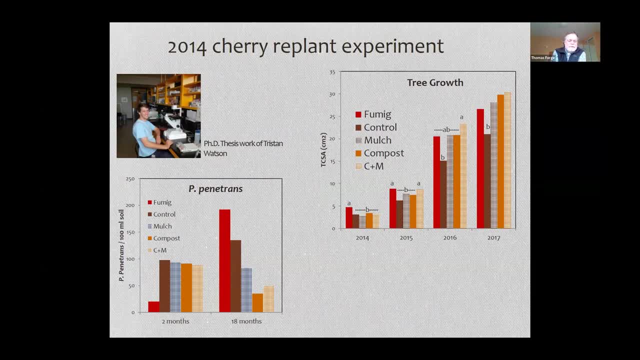 the graph on the bottom left, the very first set of bars to the left you see the red bar. So that's the nematode populations In the soil, in the fumigated plots. So very low, just residual populations left. 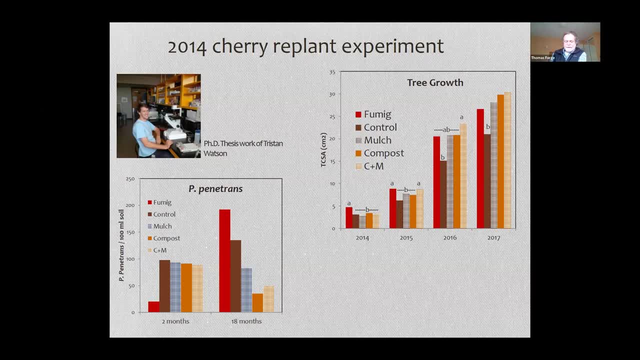 And then all the other treatments have sort of similarly high root lesion nematode population densities. The next set of bars is 18 months later And you'll notice that in the fumigated plots by that point in time they had the highest root lesion nematode population densities. 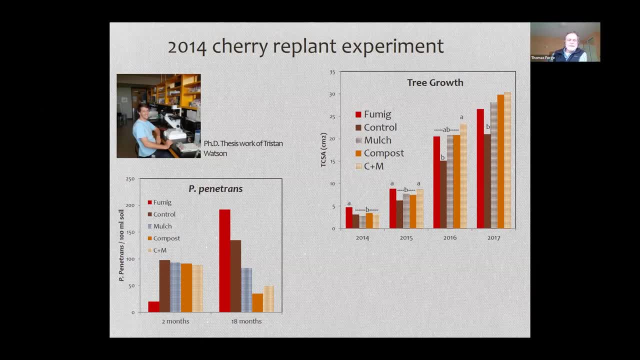 And perhaps more importantly, the lowest nematode population densities were in the plots where we had incorporated compost or where we had compost and mulch together, which were the two sort of the solid, brownish, reddish colored bar and then the hatched one to the right of it. 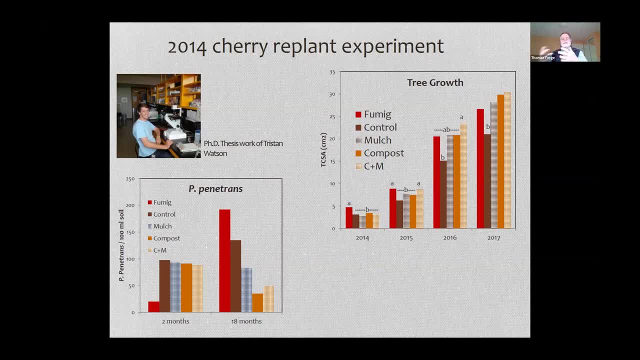 And so this is really interesting because: A it demonstrates the possibility of suppressing these organisms through time with the addition of this organic matter, But it also, kind of conversely, shows how, in the fumigated plots, we got an explosion of these nematode populations. 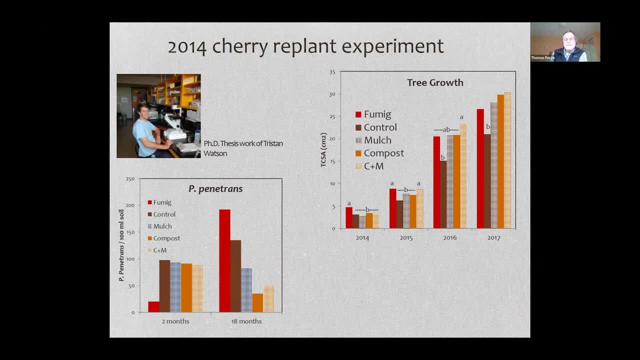 And this has been observed before in other systems- And this is due to elimination of those natural enemies that are naturally suppressing the populations. I think it's an important point to make about how soil management practices, in this case fumigation, can have deleterious effects in the long run. 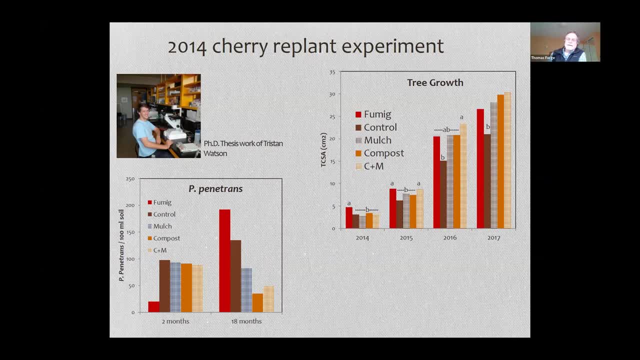 The top right-hand graph is basically trunk cross-sectional area or size of overall vigor through the years. These are the years of the experiment up through 2017.. And you see, right off at the end of the first year, the best growth was in the fumigated plots. just what we want to see. 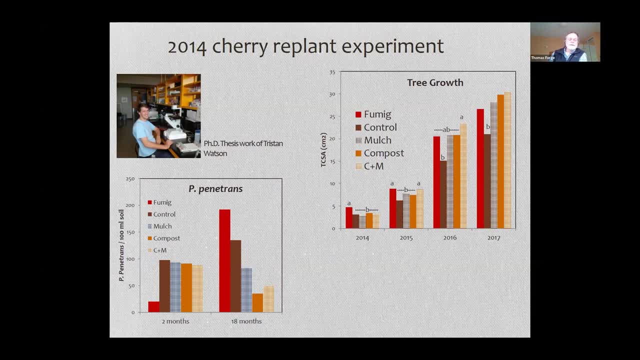 And it's actually. it's small relative to the other years, but it's significant relative to the other treatments in that year. But, as you see, in general, as the years go by, those organically amended plots rally And by the end, by 2017, they're basically starting to exceed. 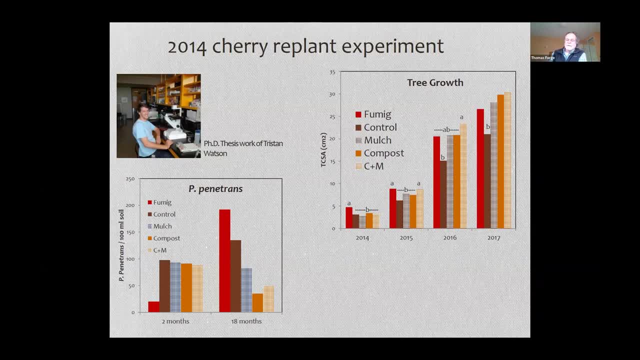 Growth in the fumigated plots showing the long-term benefits of this kind of approach- alternative to fumigation- And the PhD student we had working on this. I just want to point out that a lot of really nice work on the microbes colonizing the rhizosphere. 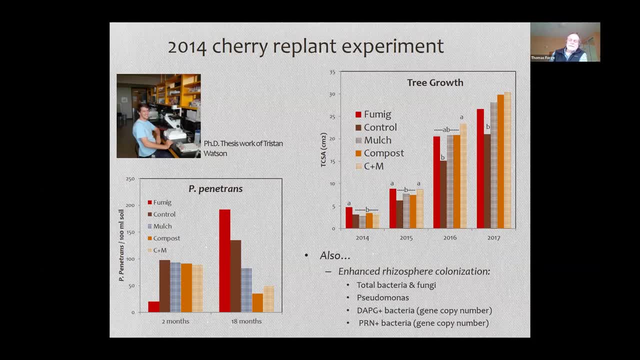 of the cherry seedlings planted in these plots and demonstrated that, with the organic amendment in this compost treatment in particular, much enhanced total populations of beneficial bacteria and fungi and in particular a group called the pseudomonads that are related to biological control in the rhizosphere. 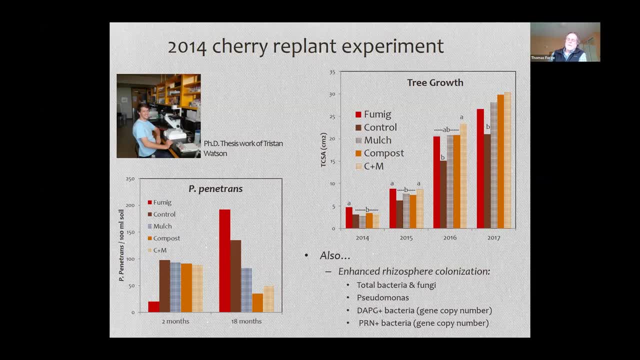 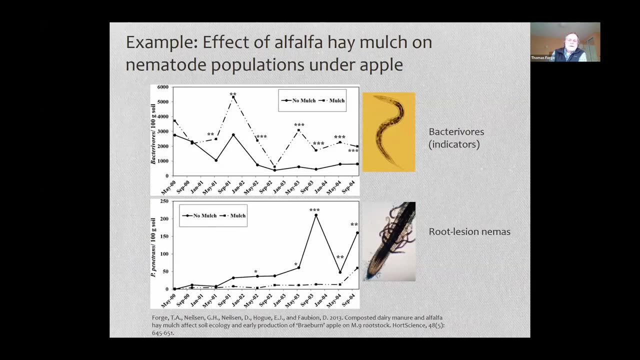 And in particular pseudomonads that are expressing genes for production of two different types of antibiotics that have been related to biological control of pathogens in the rhizosphere, and that's DAPG and PRN. So the next example I want to give you is kind of almost a hybrid between a replant experiment. 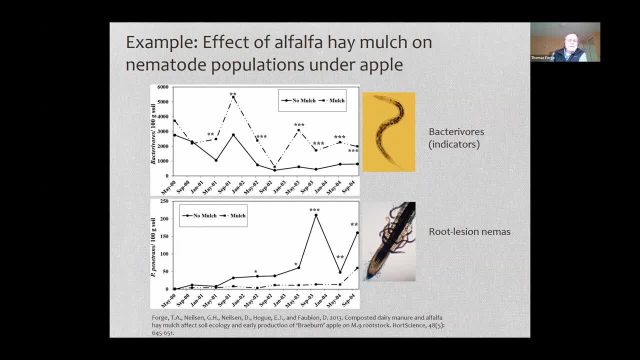 and a longer-term mulching experiment, And this experiment was done in Natchez back in the early 2000s, late 1990s, early 2000s- And what we did, and so there's quite a complex arrangement of treatments in this experiment. 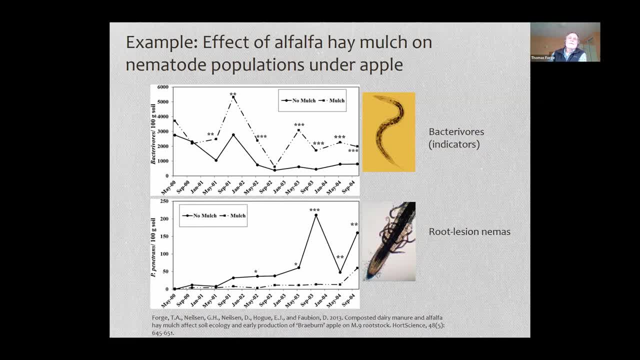 but the main ones I want to home in on right now is that there was, right after planting, there was an alfalfa mulch, alfalfa hay mulch applied and I'm comparing this to plots where we did not have an alfalfa hay mulch. 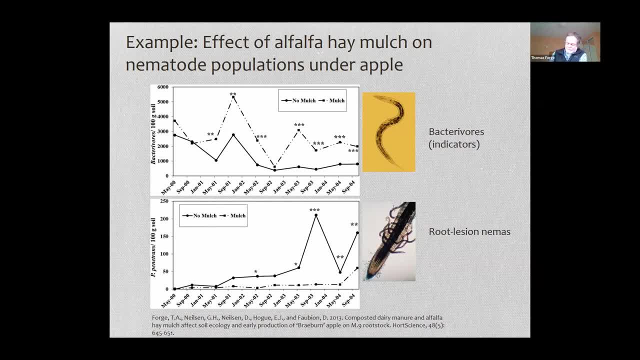 And I should point out that this block was all. it was fumigated at the beginning of the experiment. So fumigation wasn't a treatment in the experiment, but the entire thing had been fumigated, And so the top graph is populations of bacterial feeding nematodes. 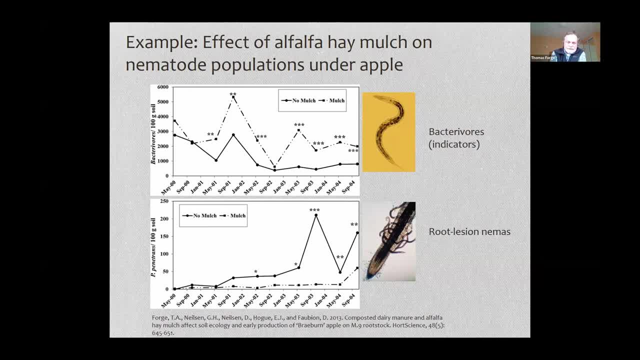 which I'm just showing you, those ones, as an indicator of overall biological activity in these soils. And you see dancing along there through the years, for the first four years, five years, the dotted line is under the mulched plots- so much higher populations of bacterial feeding nematodes. 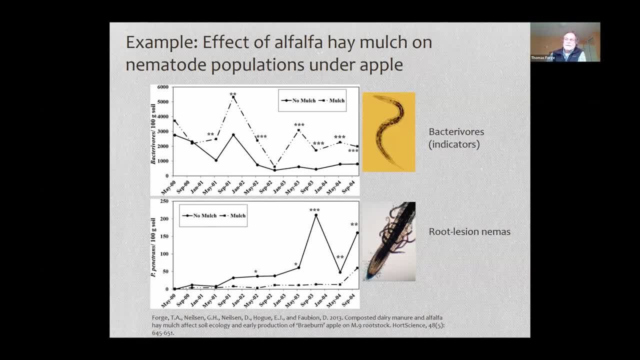 And we had similar data demonstrating increased populations of the omnivorous and predacious nematodes. It wasn't quite as consistent, but the similar trend. The bottom graph is root lesion nematode population densities in these soils and you see the complete converse of what we found with the free-living nematodes. 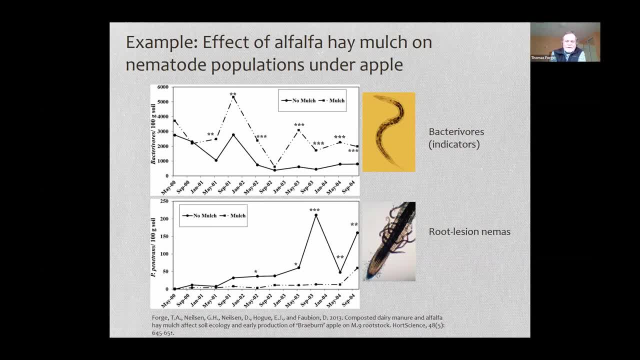 in that through time the root lesion nematode populations did come back, as we would expect in any fumigated site, but they come back much later. They come back much more rapidly and to higher levels in the non-mulched plots than in the mulched ones. 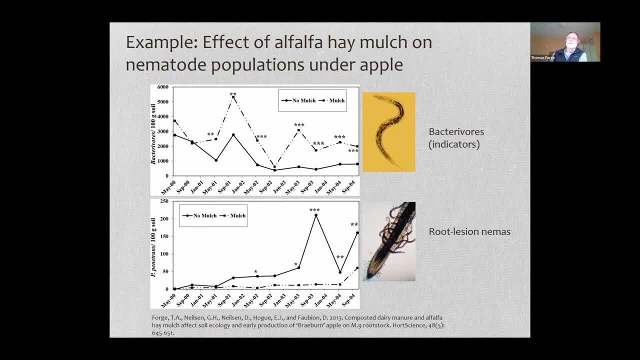 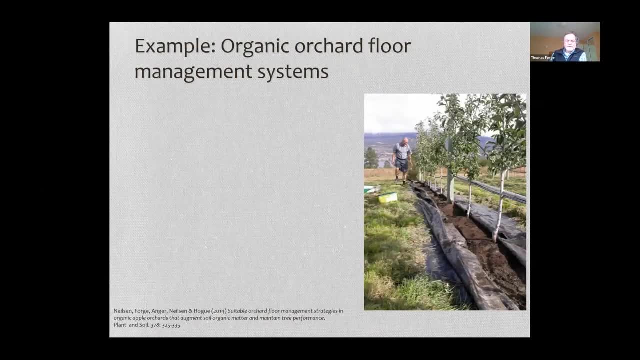 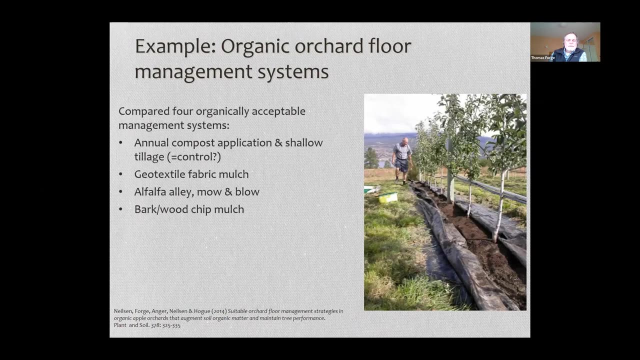 And we think this is again due to enhancement of the overall soil food web, increased populations of beneficial organisms that may be preying on or predating those root lesion nematodes. So the final example from a field experiment that I want to show you. 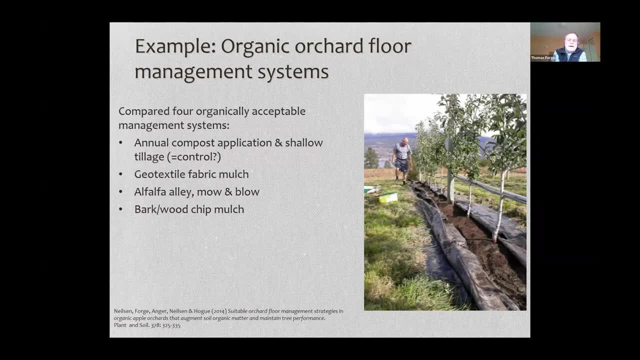 is from an experiment that we did on organically compatible orchard floor management systems up in British Columbia with Jerry Nielsen, who was the lead of this project, And this is the project that David mentioned earlier. We had four treatment options: Annual compost application with shallow tillage. 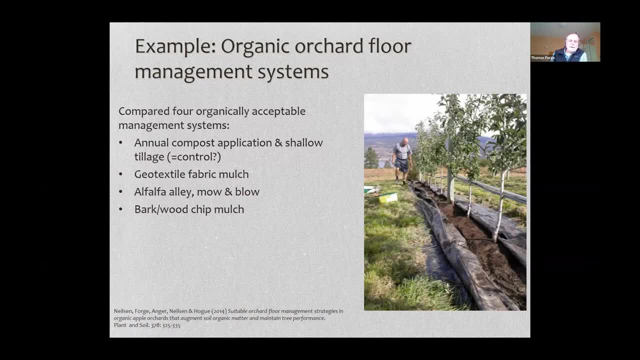 a geotextile fabric, mulch alfalfa alleyway, where we grew sorry alleyway vegetation of alfalfa primarily, and we did a mow and blow with it, And then we had the good old bark and wood chip mulch treatment as well. 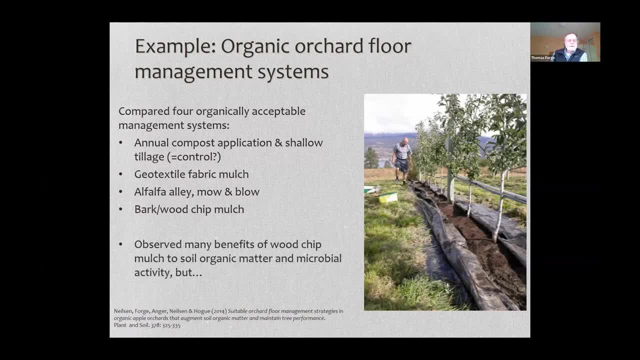 And I won't go into all the details on this, but through the years we observed many benefits, particularly under the wood chip mulch, relative to the other treatments. benefits to overall soil, organic matter, active fraction of organic matter or particulate organic matter. 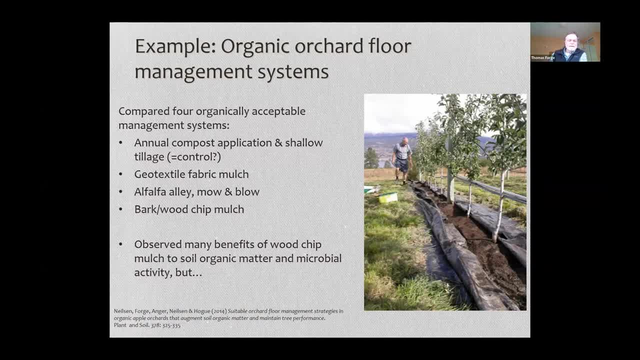 microbial activity, free living nematode, indicators of soil health, etc. But in this particular experiment we did not see any effects, suppressive effects, on root lesion nematodes, And so I point this out just to illustrate that with these kinds of systems 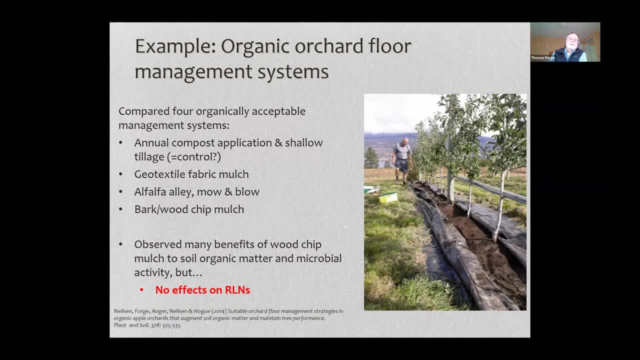 these scenarios in which we're overall improving soil health and that they don't necessarily translate to a control treatment with respect to soil borne pests and pathogens, But nonetheless, you're getting all sorts of benefits aside from that, And so it's a little bit more unpredictable. 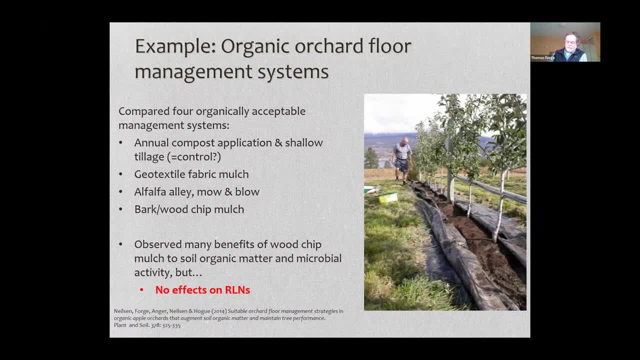 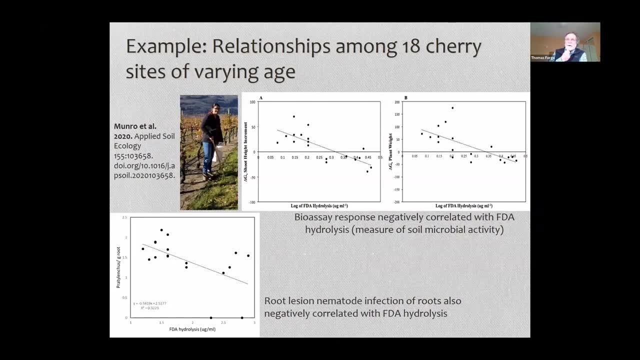 than what we typically look for for quote control management practices. But and so I kind of want to wrap up here with one last example, which is one of these correlation among sites types of examples. And so this was a graduate student, we had working with us. 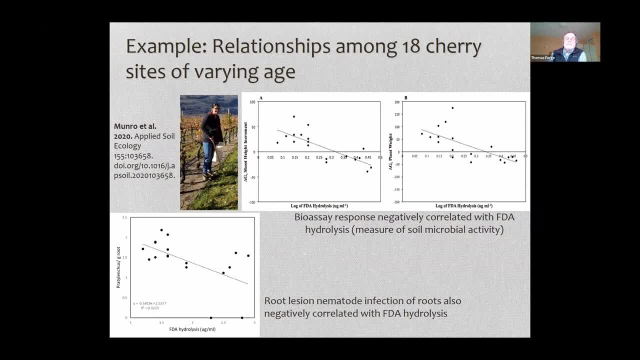 Paige Monroe, who took so much smaller in scale than Tiana's project, but 18 cherry sites up and down the Okanagan Valley, took soil, did a growth bioassay, as Tiana described for apple, And so Paige did this with cherry. 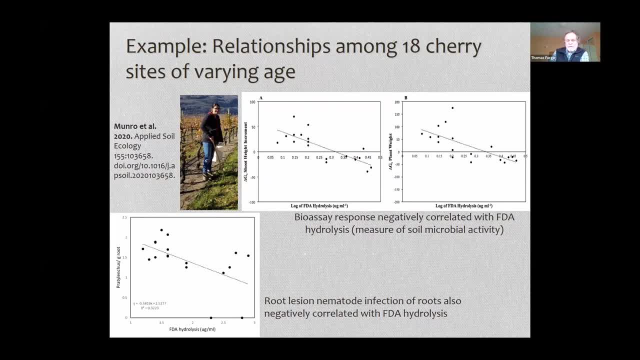 The growth bioassay, And then she also, on those soil samples, measured a whole bunch of soil properties, including indicators of soil biological activity and pox carbon as indicators of soil health. And so the graph, the two graphs on the top right that you see. 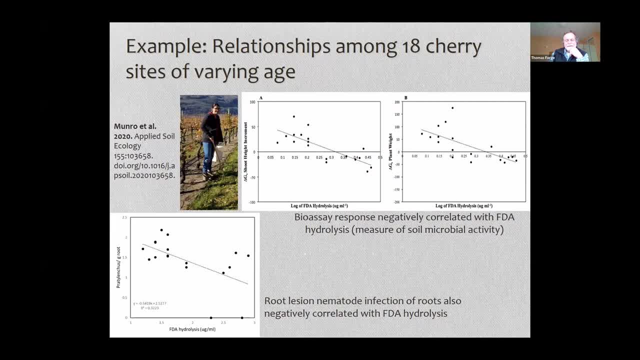 on the x-axis is a measurement of fluorescein diacetate activity, which is basically an indicator of microbial activity, And the two different graphs. one of them is for plant weight, overall plant weight in the bioassay and the other one is for shoot height. 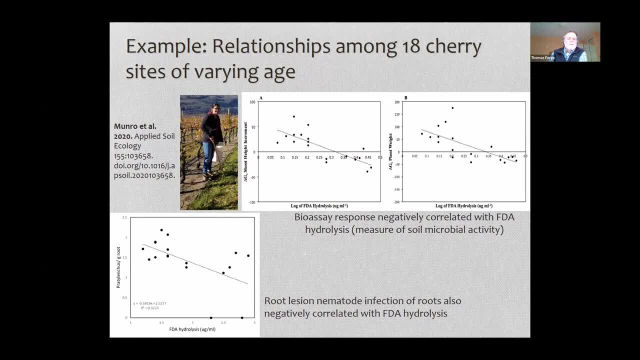 So they're pretty comparable And they both get at the same thing, And so what I want you to so in the interpretation of this is: towards the left you see all the high sites. So those are sites or soils where there was a significantly positive response. 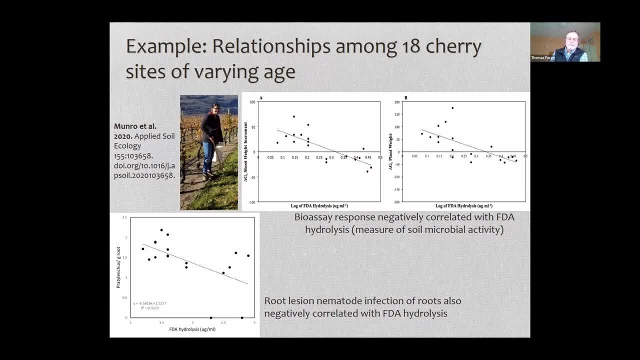 to pasteurization of the soil or improvement in growth due to pasteurization. So these were sites where there was a lot of pathogen pressure, But then, as you move to the right sites that had higher levels of overall microbial activity, you actually had the opposite. 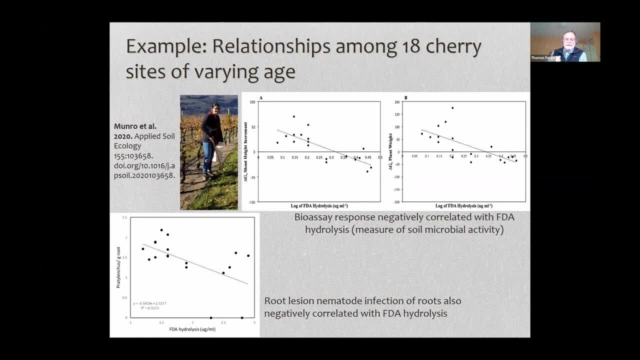 where pasteurization, if anything, decreased growth of the trees. So this is illustrating the relationship between overall soil biological activity and essentially pathogen pressure. But then also we have the same relationship down the bottom left between fluorescein, diacetate hydrolysis. 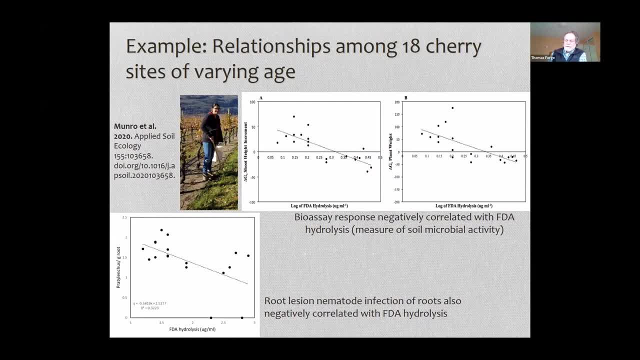 as we're just describing, and the degree to which the roots in those bioassay plants were colonized by these root lesion nematodes. So that's an infield or a cross-site demonstration of some of these relationships that we expect to see. 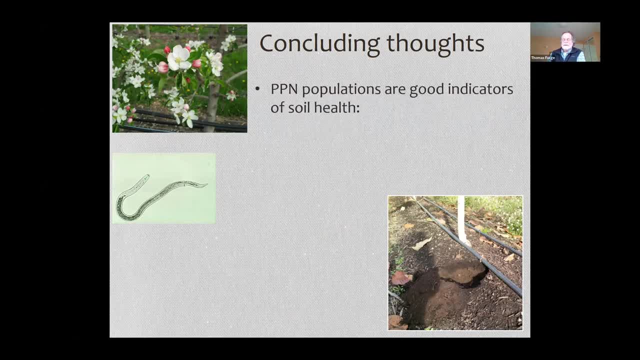 So just concluding thoughts on plant parasitic nematodes. They are good indicators of soil health or, to put it another way, they should be considered as one of the many things that we can measure as a comprehensive assessment of soil health. This is largely because they are direct determinants. 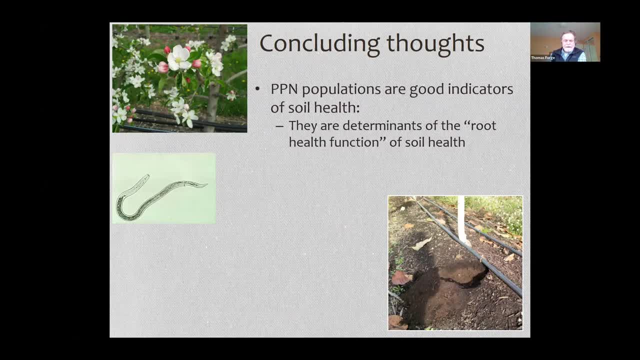 of the root health function of soil health. They directly affect root health And their population densities can be correlated with yields and packouts And we're starting to get a little bit better handle on this. We didn't have a lot of information along these lines. 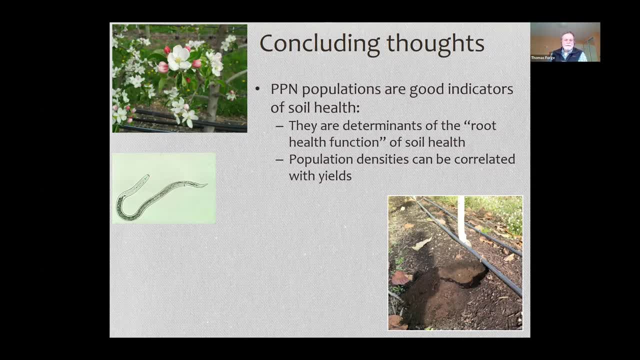 but Tiana's big soil health study, Paige's recent study and various others are starting to point in this direction that it is possible to directly relate. But also soil organic matter management practices can suppress root legion nematode populations.